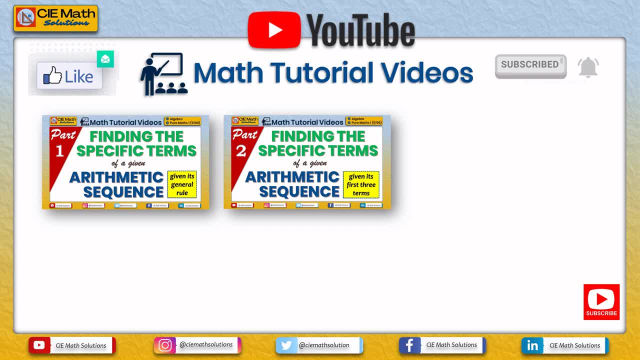 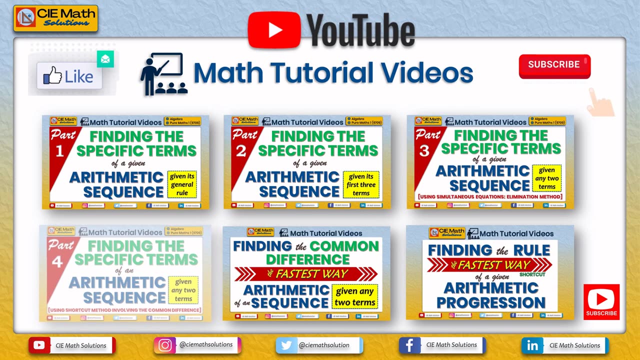 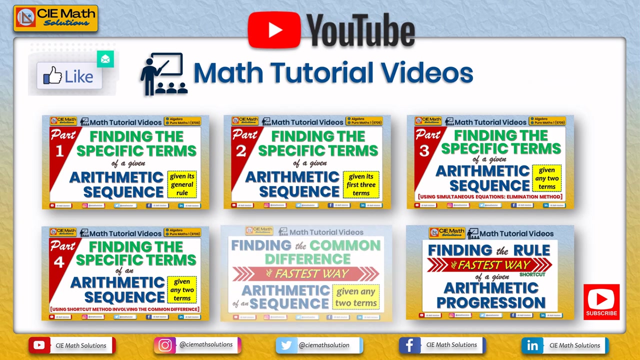 terms. We have also explored the use of simultaneous equations in finding the specific terms of a given arithmetic sequence. The playlist containing these videos, together with other math tutorial videos about sequences and series, are found on the link above this video or in the description below. If you are new to this channel, please consider subscribing. 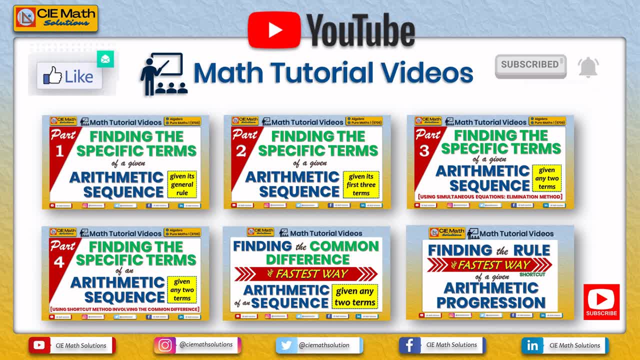 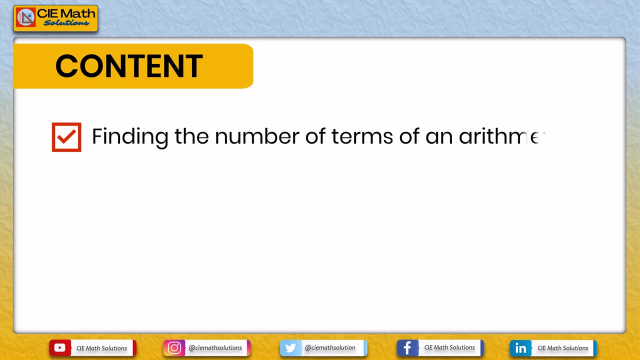 and don't forget to hit the bell icon for you to be notified when new videos are uploaded. If you have already subscribed, please watch, like and share the videos of the channel. Thank you. 2 Steps in this video we will focus on finding the number of terms of an arithmetic sequence. 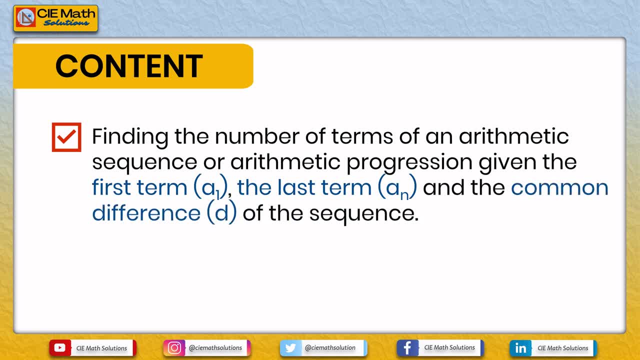 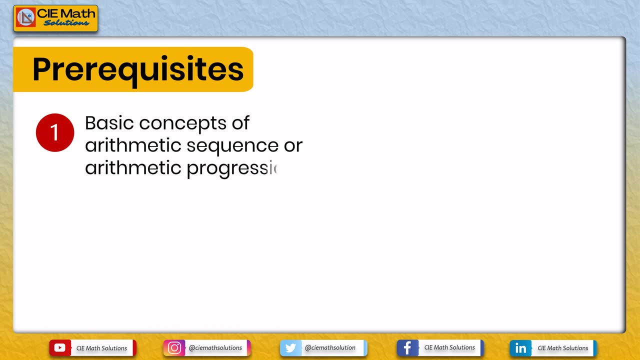 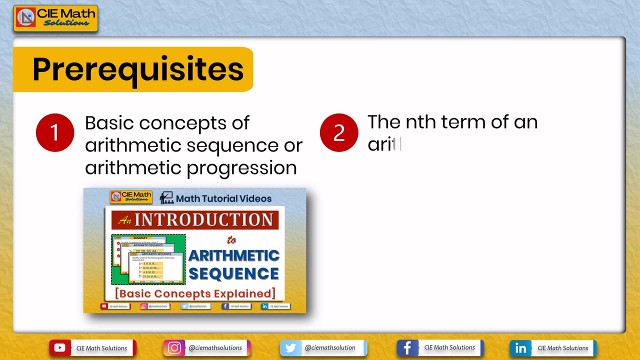 or arithmetic progression, given the first term, the last term and the common difference of the sequence. but before we proceed, let us have a quick recall of the prerequisite concepts needed. first, the basic concepts of arithmetic sequence or arithmetic progression. Second, the nth term formula of an arithmetic sequence. 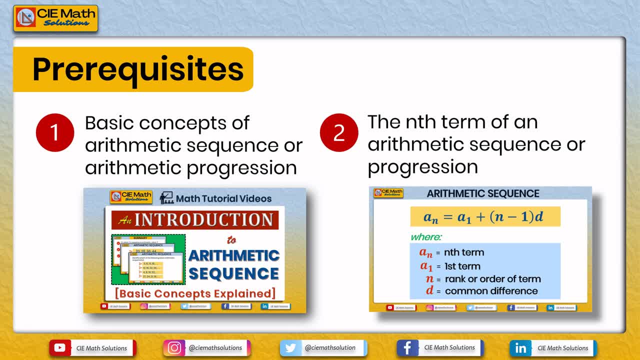 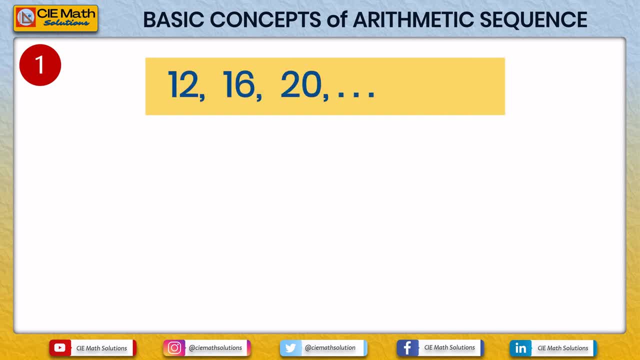 or progression. For the first prerequisite, given an arithmetic sequence containing the terms 12,, 16, and 20,, the numbers 12,, 16, and 20 are called the terms of the sequence and they are usually denoted by a n In this case. then, 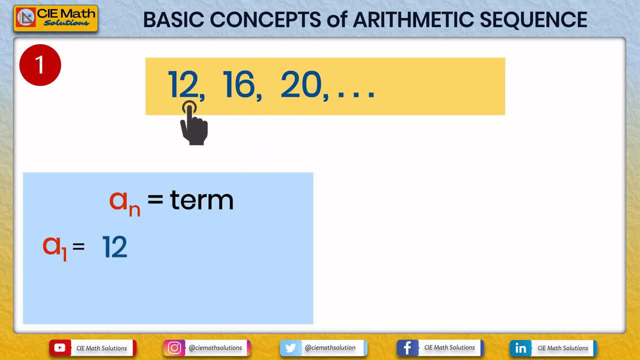 a1, which is the first term, is 12,. a2, which is a second term, is 16,. a3, which is the third term, is 20.. The arithmetic sequence also has a common difference, which is denoted by d. d here is equal to 20 minus 16 or 16 minus 12.. The difference: 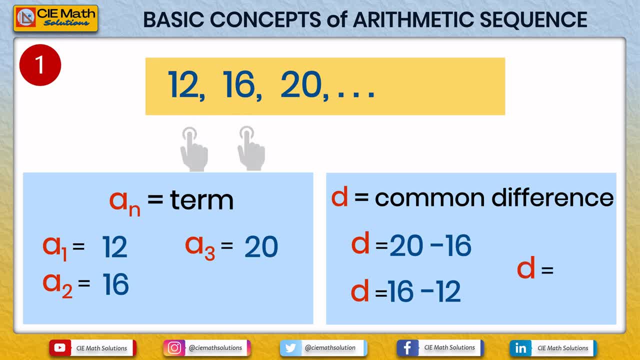 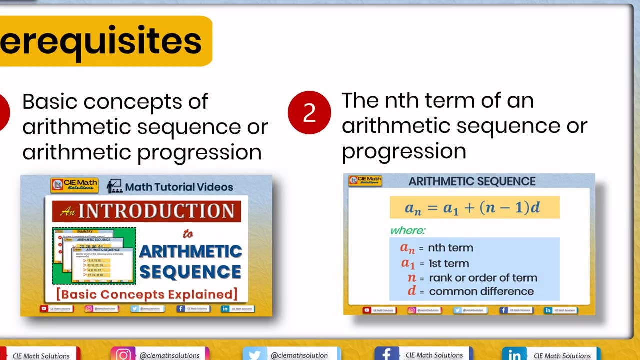 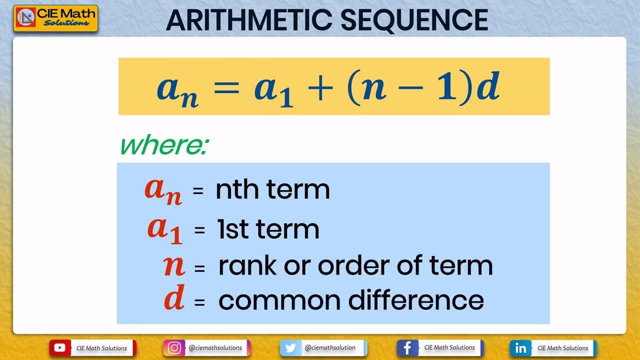 of these are the same, which is equal to 4.. The common difference, then, of this arithmetic sequence is equal to 4.. For the second prerequisite concept, the nth term formula of an arithmetic sequence is a: n equals a1 plus n minus 1 times d a n. here is the nth term. a1 is the first term. 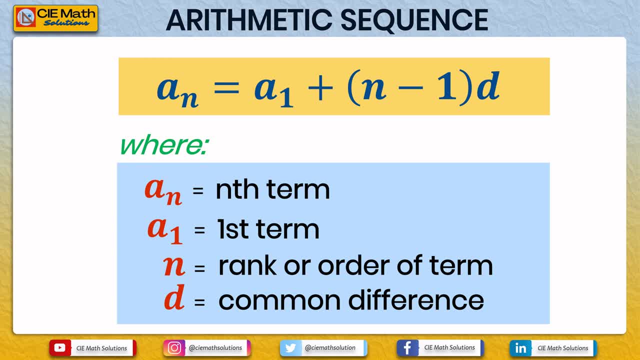 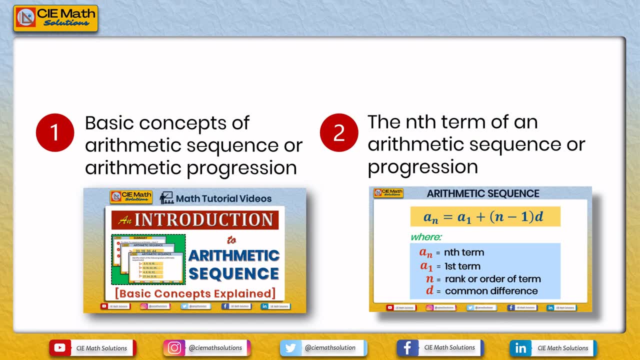 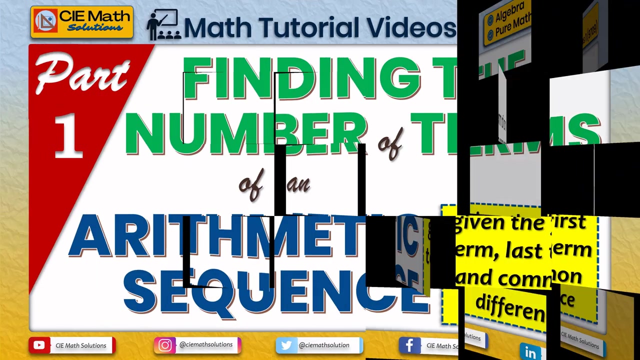 n is the record order of the term And d is the common difference. If you would like to study more about these prerequisite concepts, you may click the link above this video or in the description below. Not let us use these prerequisite concepts in finding the number of terms of an arithmetic. 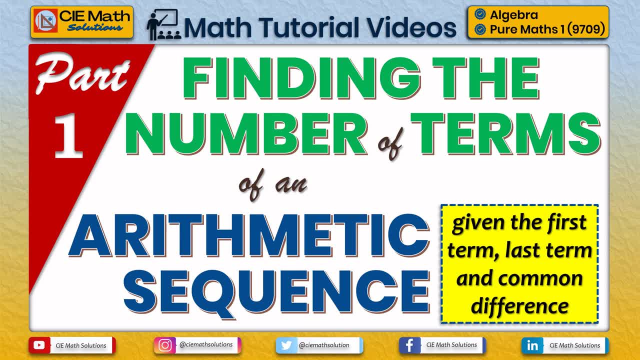 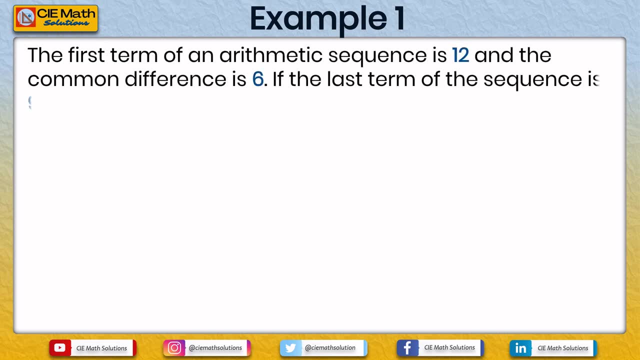 sequence or progression given its first term, last term and common difference. For example, the first term of an arithmetic sequence is 12 and the common difference is 6.. If the last term of the sequence is 90,, how many terms are there in the sequence? 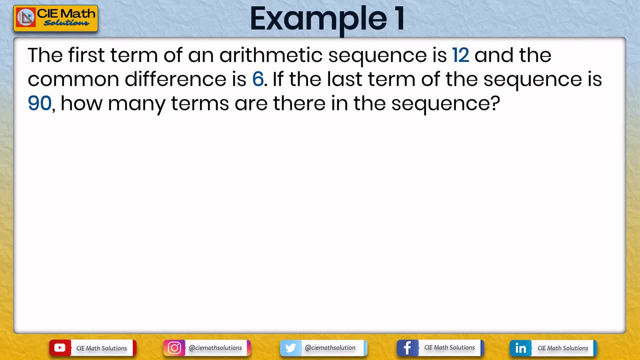 Before we could find the number of terms of the given arithmetic sequence, let us summarize first all the given data: a1. Before, the first term is 12,. a, n, or the last term is 90, and d, or the common difference is 6.. 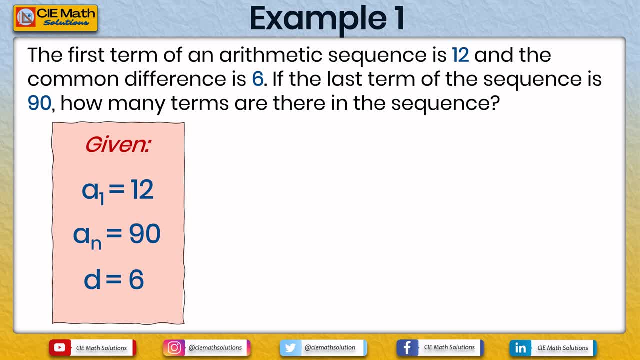 To find the number of terms we will be needing the nth term formula of an arithmetic sequence: a- n is equal to a1 plus n minus 1 times d. Let us then substitute the given in this formula. We already have a, n, a1, and d. 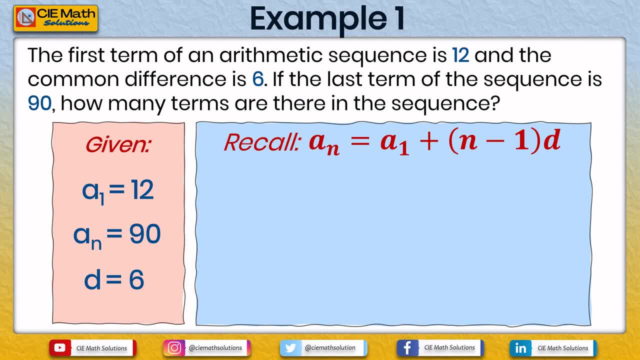 So the equation then will become 90 equals 12 plus n minus 1 times 6.. Distributing 6 to n minus 1, we then will have 90 equals 12 plus 6n minus 6.. Simplifying the equation further, we will then have 90 minus 12 plus 6 equals 6n, ie. 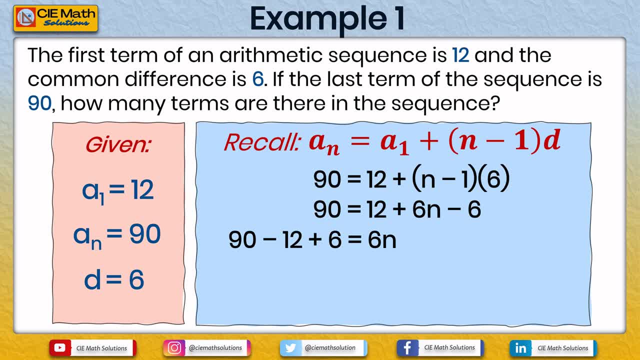 moving all the constants on the left side For each of the dies owe to gra, acomplishing the result. Steph problem in this video may ヽ: the left side. simplifying the left side: 90 minus 12 plus 6 is equal to 84 that. 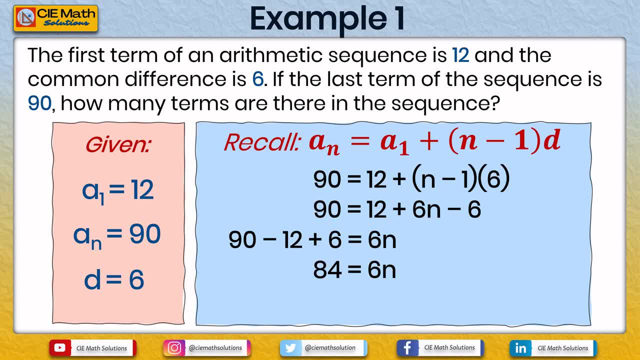 is equal to 6n. dividing both sides by 6, we will then have the value of n, which is equal to 14. therefore, there are 14 terms in the arithmetic sequence with a common difference of 6, with first term 12 and last term 19. 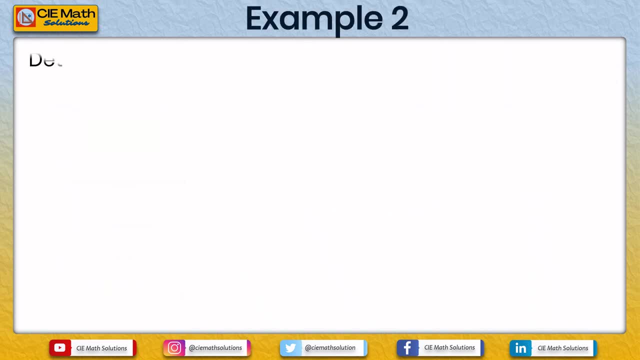 for the second example, determine the number of terms in the following arithmetic sequence: 27, 35, 43, 51, dot, dot, dot, 195. let us identify first the given. in the sequence, the first term is 27 and also the last term is 195. in this case, the common difference is not given, however. 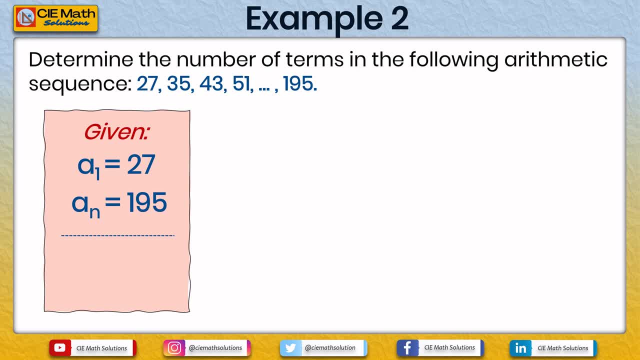 we know that in an arithmetic sequence the common difference is the difference between consecutive terms of the sequence. we can then subtract 35 minus 27, which will give us 8. take note that you can subtract any two consecutive terms. you will also get 8 if you subtract 43 and 35. the same case if. 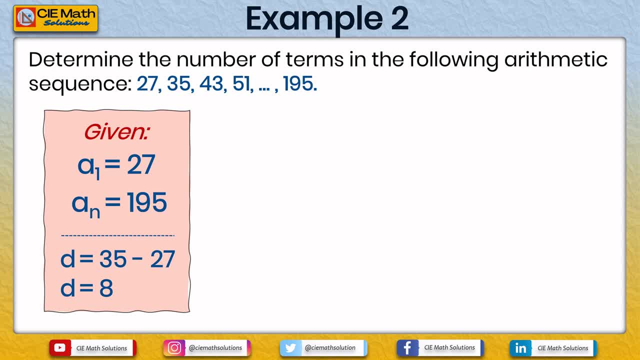 you subtract 51 and 43, the value of the common difference will still be 8. substituting this, given now to the end-term formula, we will then have: 195 is equal to 8.5, is equal to 1.5, and Sean also says that number of terms is equal to 23.5.. 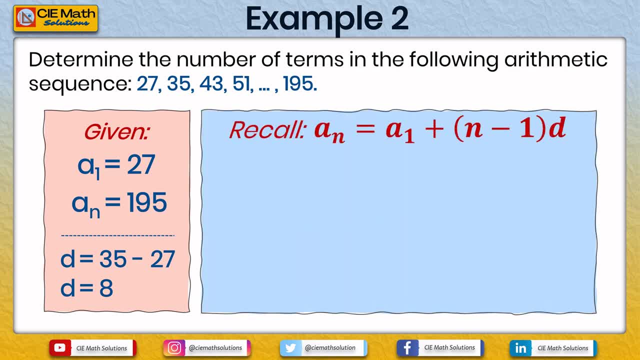 this, given now to the end-term formula we will then have: 195 is equal to 22 and we have some to 27 plus n minus 1 times 8.. Simplifying the equation further, 195 is equal to 27 plus 8n minus 8.. And simplifying the constants, or combining those constants: 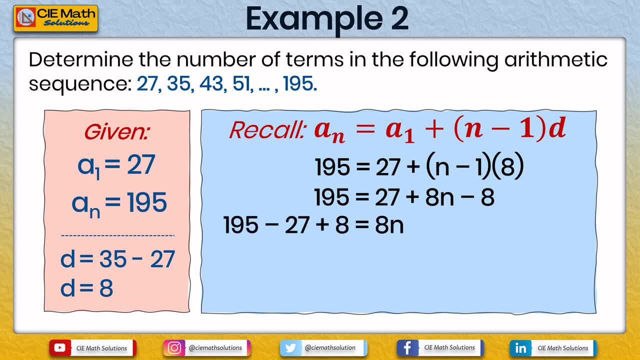 we will then have 195 minus 27 plus 8 is equal to 8n, which is equal to 176.. Dividing both sides by 8, we will then have n equals 22.. Therefore, there are 22 terms in this arithmetic sequence with a common difference of 8, first term 27 and. 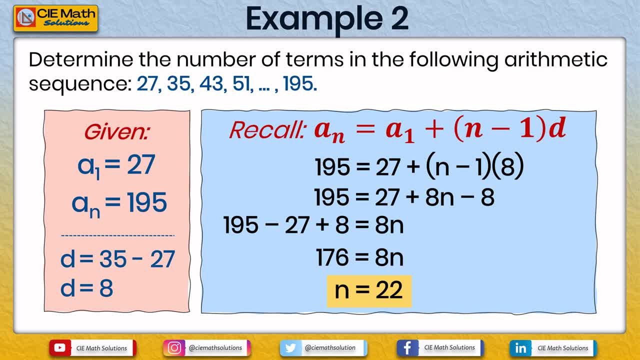 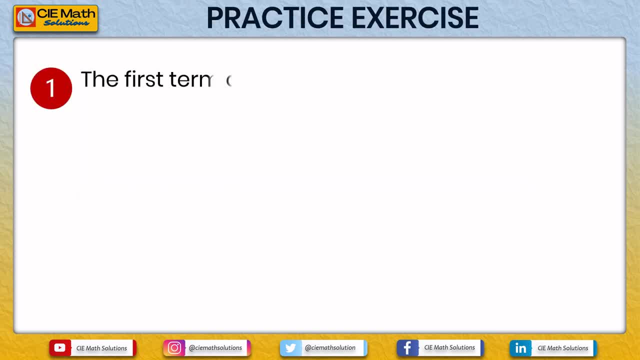 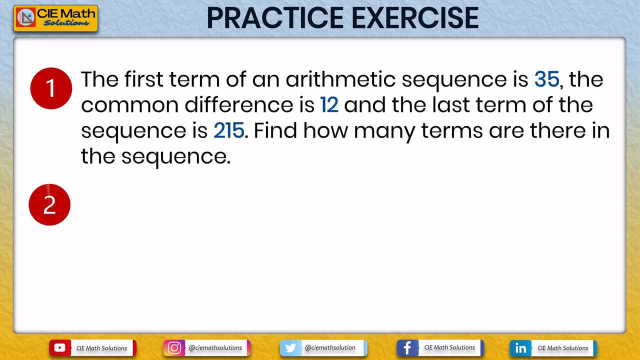 last term, 195.. Now it's your turn. The first term of an arithmetic sequence is 35,. the common difference is 35.. And the last term of the sequence is 215.. Find how many terms are there in the sequence. Determine the number of terms in the following arithmetic sequence: 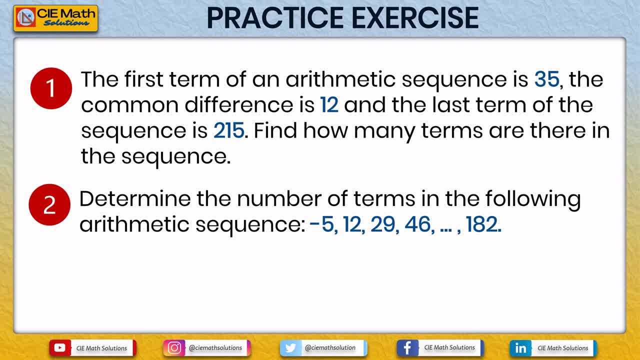 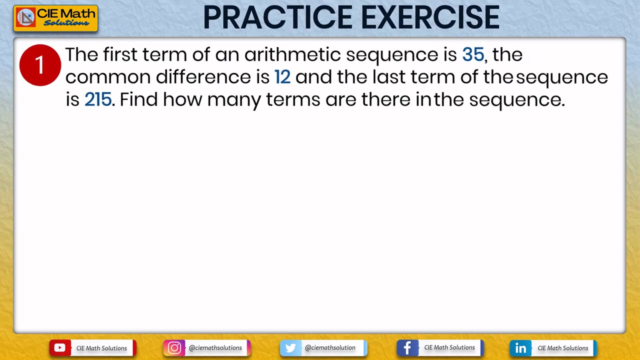 negative: 5,, 12,, 29,, 46,, dot, dot, dot. 182.. If you would like to try to answer these items, please pause the video for a while And when you're done, press the play button now. Now let us have the answers. Starting off with the first item, let us summarize the. 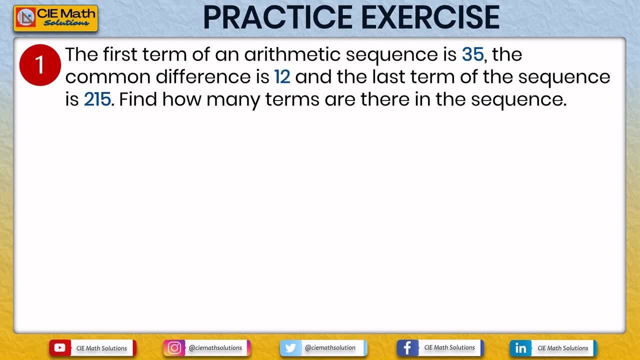 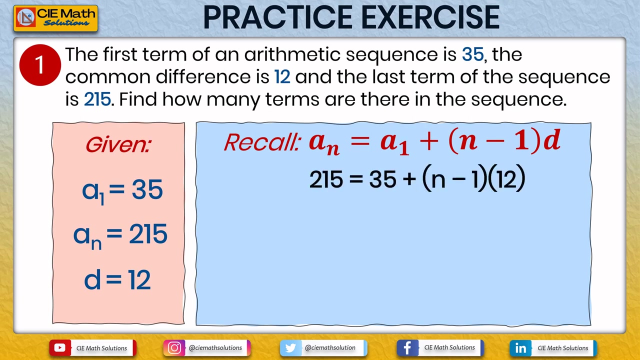 given data. First, the first term is 35,, the last term is 215, and the common difference is 12.. If we substitute these values to the n-term formula of an arithmetic sequence, we will then have: 215 is equal to 35 plus n, minus 1 times 12.. Simplifying this equation: 215. 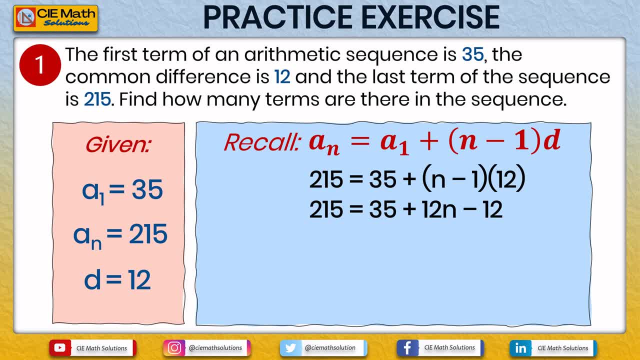 equals 35 plus 12n minus 12.. We will then have: 215 minus 35 plus 12 is equal to 12n, which is equal to 192.. Dividing both sides by 12,, the value then will be 16.. Therefore, there are 16 terms. 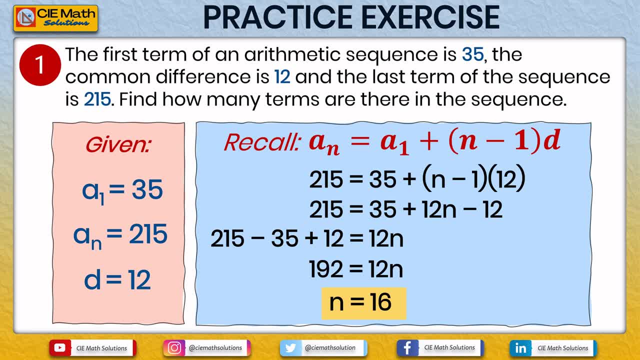 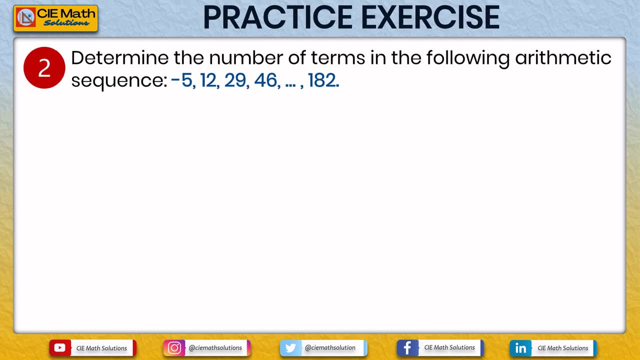 in this arithmetic sequence with a common difference of 12,, with first term 35 and last term 215.. For the second item, determine the number of terms in the following arithmetic sequence: negative: 5,, 12,, 29,, 46,, dot, dot, dot, 182.. If you would like to try this, please pause. 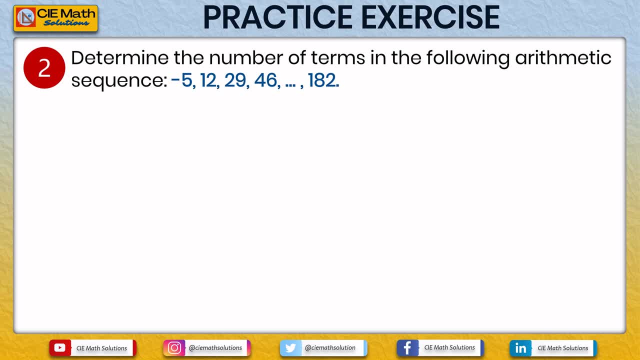 the video for a while Again. let us first MORE than it out and look at 0.. See here my comment is wrong. The picture is good, which means this is correct. The second time we will get an equation of 12,, 19,, 46, and we can surprise the fifth. 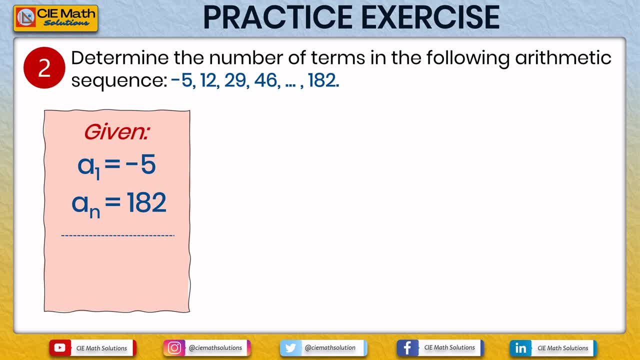 one by multiplying these twohape by 12.. Okay, so we have 12 minus 19,, 47,, which is equal to 1.. We will subtract both of these times, So the first term here is negative 5, and the last term is 182. 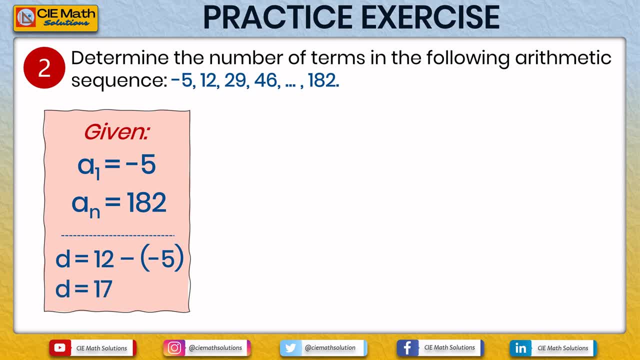 The second term is wise enough to be used toelavers. The last term is 282.. if we subtract 29 and 12, the same case 46 and 29.. Substituting these values on the n-term formula, we then have 182 equals negative 5 plus n minus 1 times. 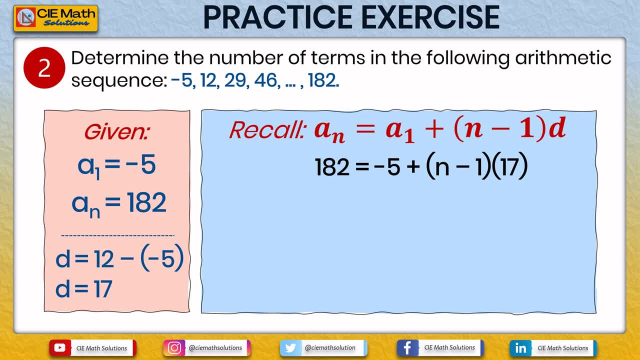 17, which is equal to 182, equals negative 5 plus 17n minus 17.. Combining the constants, we have: 182 plus 5 plus 17 equals 17n. That is equal to 204.. Dividing both sides by 17,, we will then have n equals 12.. The number of terms: 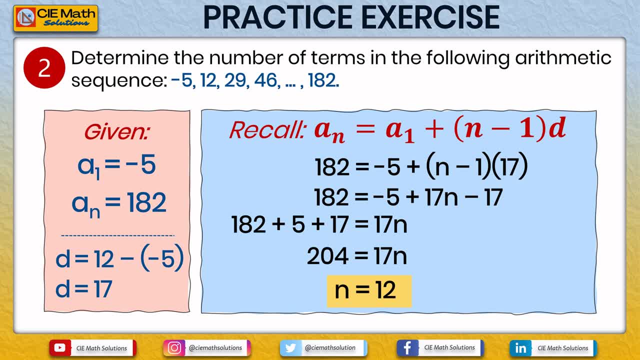 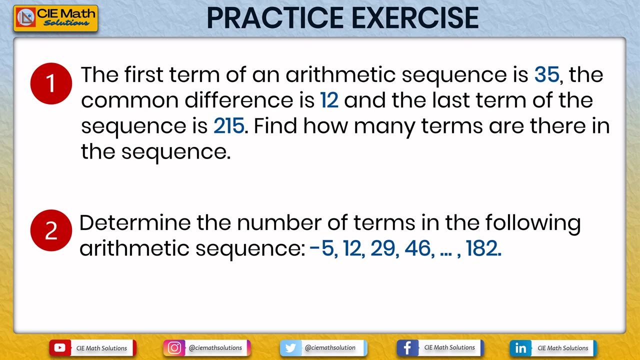 then in this arithmetic sequence, with a common difference of 17, with first term negative 5 and last term, 182 is equal to 12.. Summarizing the answers of the items, the number of terms in the first item is 16 and the number of terms in the second item is 12.. If you got the answers, 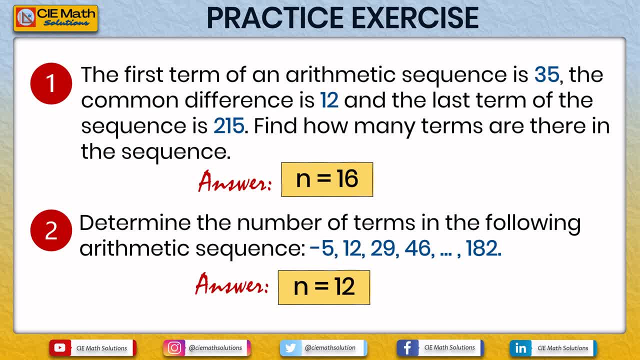 correct, then congratulations. You now know how to find the number of terms of an arithmetic sequence or progression, Given the first term, last term and the common difference. If you did not get all the answers correct, don't worry, You can still practice for more. You may also: 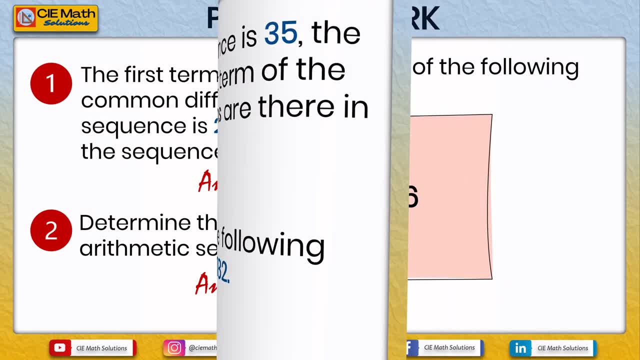 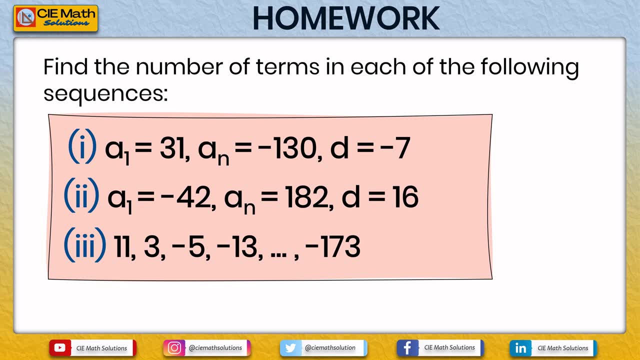 answer the following homework. Find the number of terms in each of the following sequences. First: a1 is 31,, an is equal to negative 130, and d is equal to negative 7.. Second: a1 is negative 42,, an is 182, and d is equal to 16..